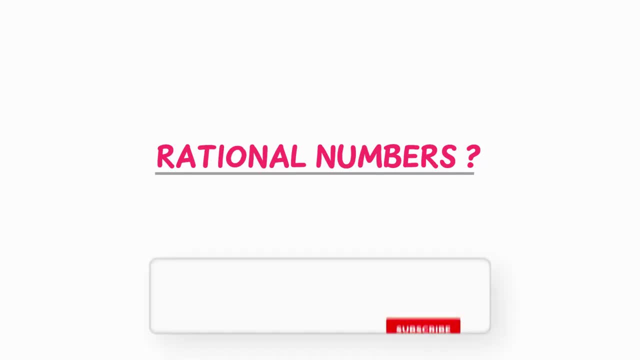 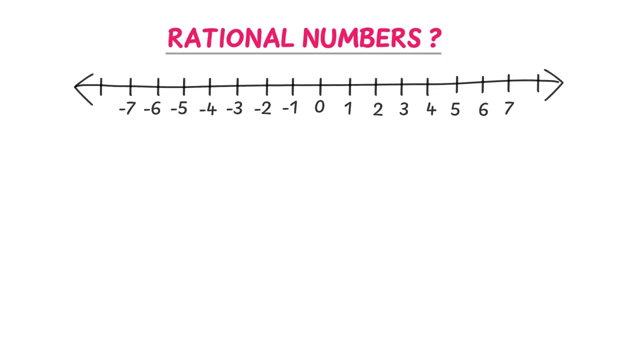 What are rational numbers? Before starting the lecture, click on the subscribe button and get access to our hundred of conceptual lectures for free. Now understanding the easy concept of rational numbers. We have learned all about the number line and real numbers in the previous video. 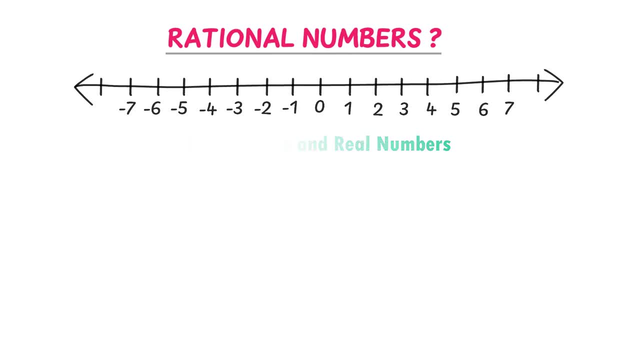 If we pick up any two integers from the number line and put them into fraction or p by q form- except q shouldn't be equal to 0,- we get a rational number. For example, consider a 1.. We know that 1 can be written as 1 divided by 1.. 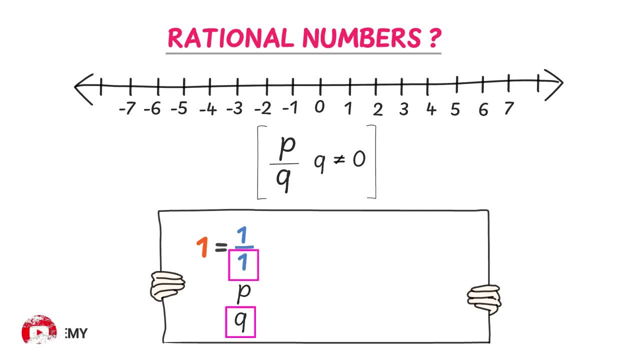 It is a p by q form where q isn't equal to 0.. So 1 is a rational number. Consider a 6.. We know that we can write 6 as 6 divided by 1.. It is a p by q form where q isn't equal to 0.. 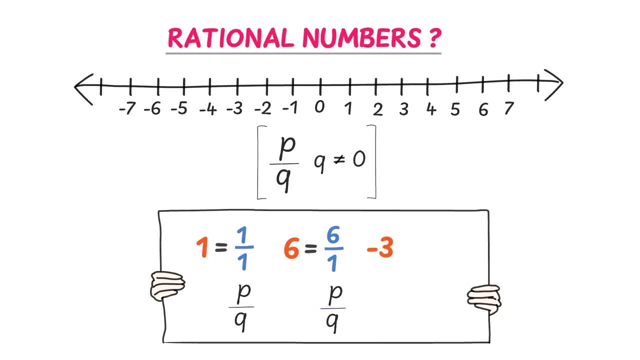 So it is also a rational number. Consider a minus 3.. We can write minus 3 as minus 3 divided by 1.. It is also a p by q form, So it is also a rational number. From this example we learn that all positive integers and negative integers are rational numbers. 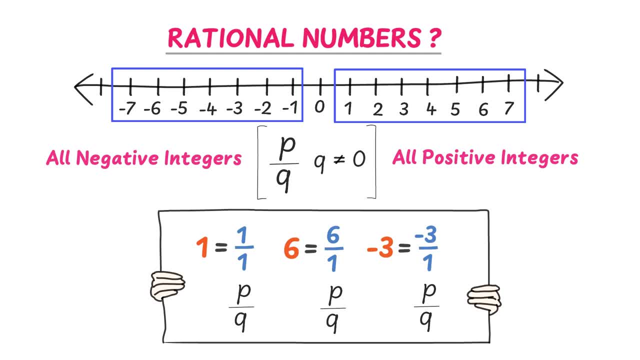 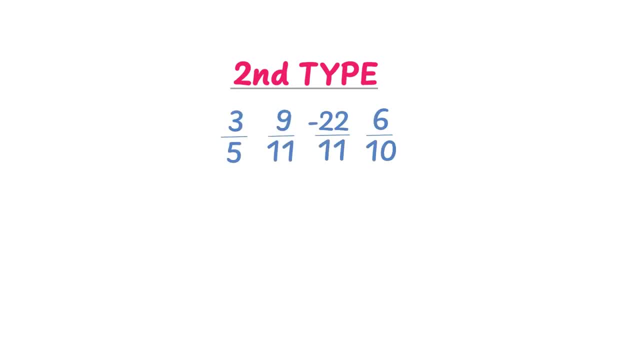 Let me repeat it: All positive integers and negative integers are rational numbers. The second type of rational numbers is like 3 divided by 5, 9 divided by 11, minus 22 divided by 11, 6 divided by 10.. 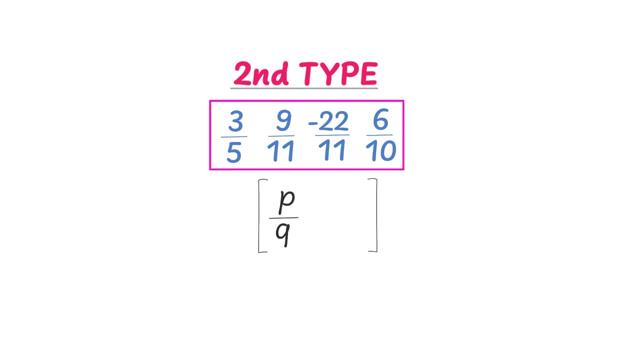 Remember that all these numbers are in p by q form where q isn't equal to 0.. For instance, 3 as a numerator is a positive integer and 5 as a denominator is also a positive integer. So this number is in the p by q form where q isn't equal to 0. 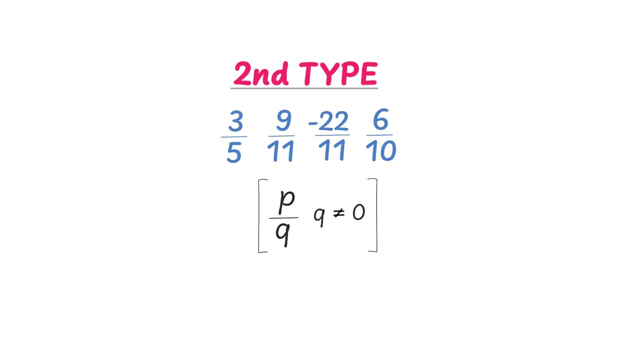 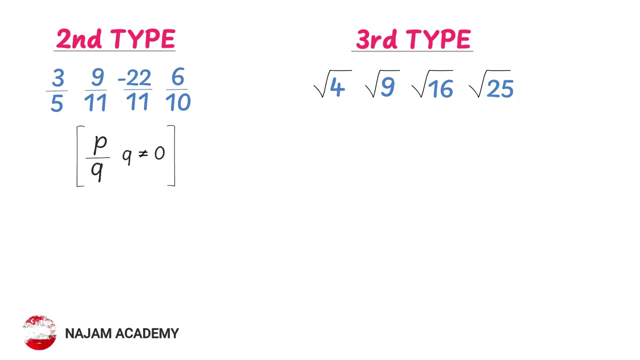 Thus it is a rational number. Therefore we say that such type of numbers are rational numbers. The third type of rational numbers are like root 4, root 9, root 16 and root 25.. We know that the square root of 4 is 2.. 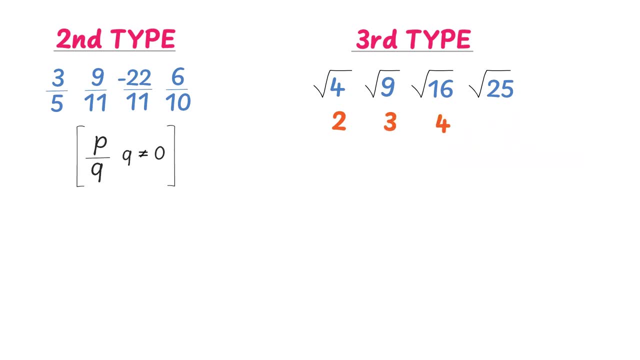 The square root of 9 is 3.. The square root of 16.. The square root of 17 is 4. And the square root of 25 is 5.. We also know that all these numbers are positive integers And we can write them in fraction or p by q form. 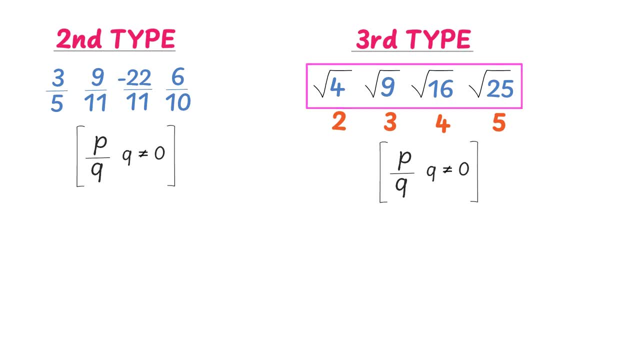 Thus all these numbers are also rational numbers. The fourth type of rational numbers are 4.6666, and so on, 3.5,, 2.515151.. And so on, 4.67, etc. Now, 0.6666 is an example of non-terminating and recurring decimal number. 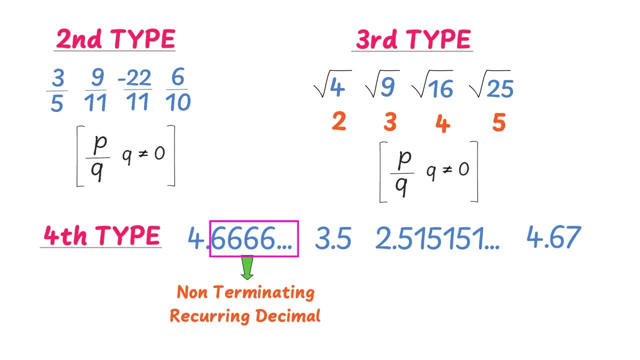 Because the digit 6 repeats itself in the decimal part and it is non-terminating. Remember that such type of numbers having non-terminating and recurring decimal part are rational numbers Like 2.55.. 515151.. Secondly, 3.5 is an example of terminating decimal. 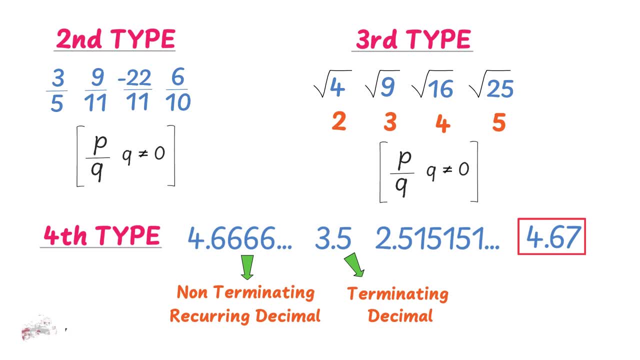 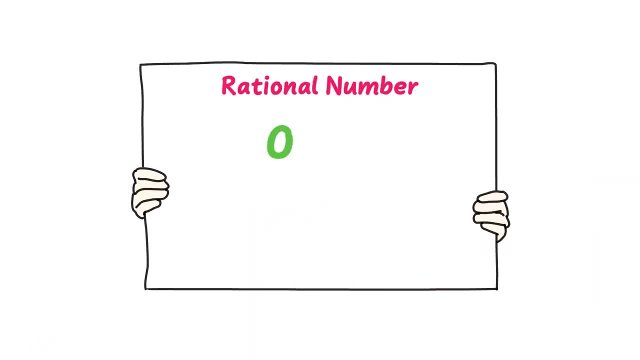 All such type of numbers, like 4.67, are also rational numbers. Finally, as a bonus tip, remember that 0 is a rational number Because we can write it in a fraction, or p by q form, As 0 divided by 1.. 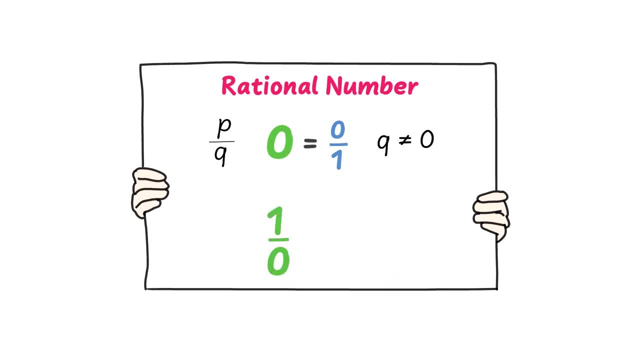 Where q isn't equal to 0. But 1.. Divided by 0 is not a rational number, Because here q is equal to 0. We know that 0 divided by 1 is equal to 0.. And 1 divided by 0 is undefined or it goes to infinity. 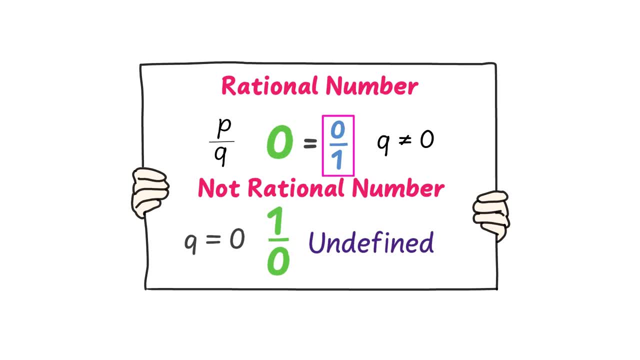 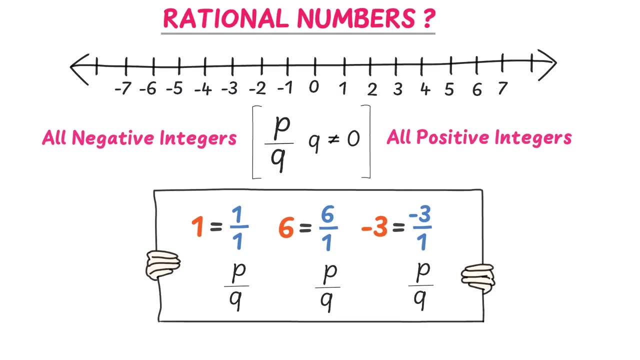 So we therefore say that 0 divided by 1 is a rational number And 1 divided by 0 is not a rational number. To summarize my lecture, we learn that all positive integers and negative integers are rational numbers And negative integers are rational numbers. 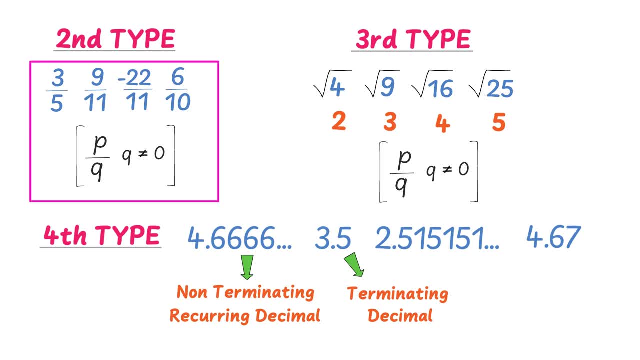 Secondly, we learn that all numbers that can be written in the p by q form are rational numbers. Thirdly, all numbers like square root of 4, square root of 9, square root of 16 are rational numbers. Finally, we learn that all numbers having non-terminating and recurring decimals are rational numbers.